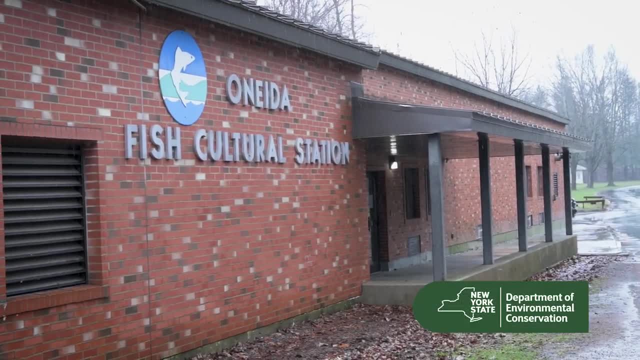 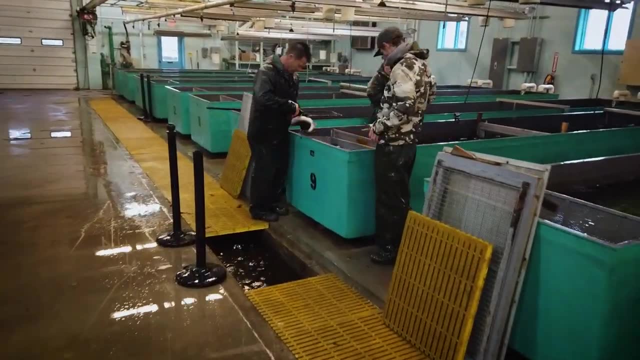 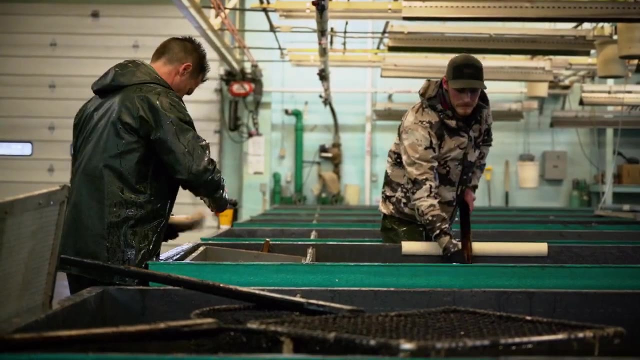 Cornell is contracted through DEC to study a night a lake. so they're the ones that get the population estimates on the lake for the various species. so this is a great opportunity for them to come in. we have a lot of fish on hand. we go through a lot of fish so they can mark the fish. 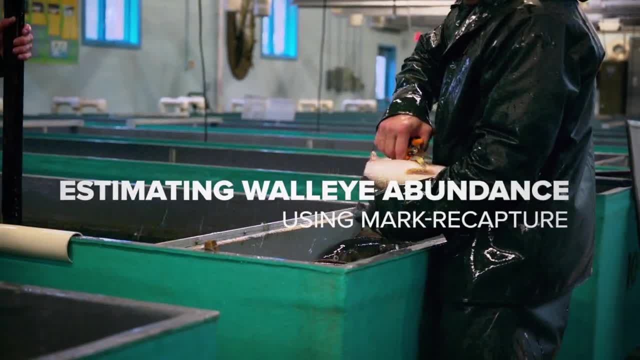 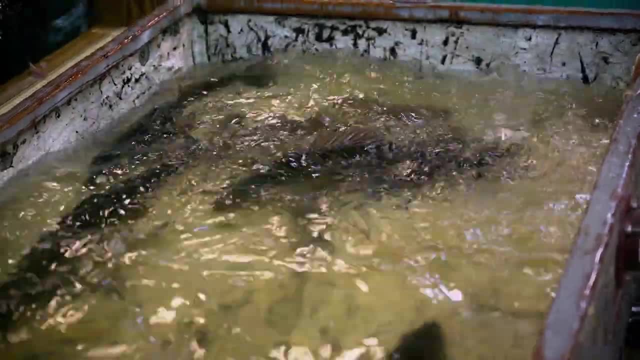 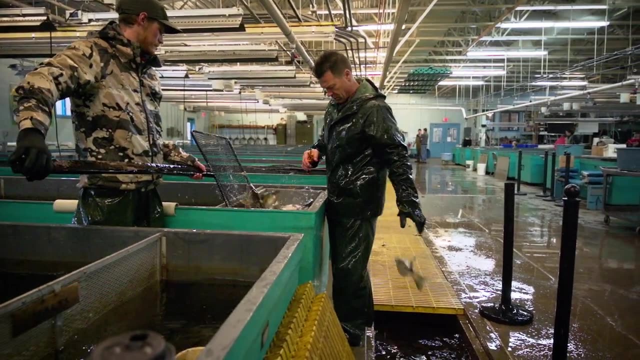 they need to and use those marked fish to extrapolate the number of fish in the lake when they recapture them throughout the summer when they're netting. I'm Tony Vandevalk at Cornell University. I'm a research support specialist, whether you're an angler, researcher or a fish. 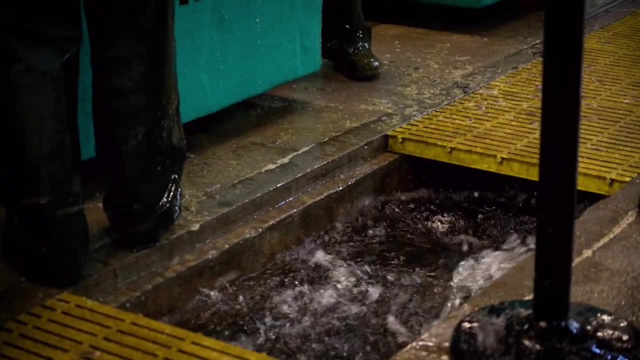 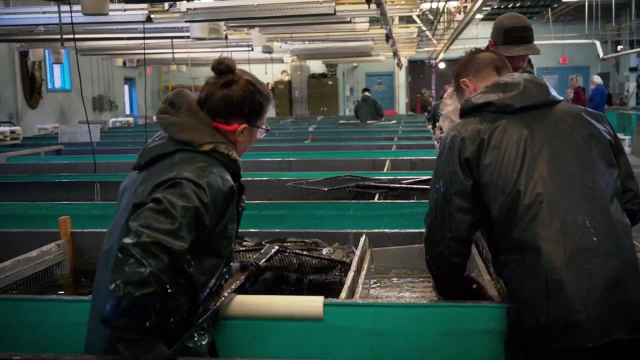 manager, one of the most valuable pieces of information you can have on a system are the number of fish that are in the lake. One way to do that is through a marker capture experiment. a marker capture experiments are very labor-intensive and they require you to mark a lot. 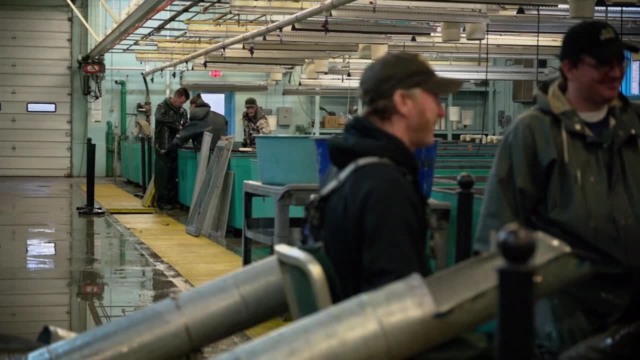 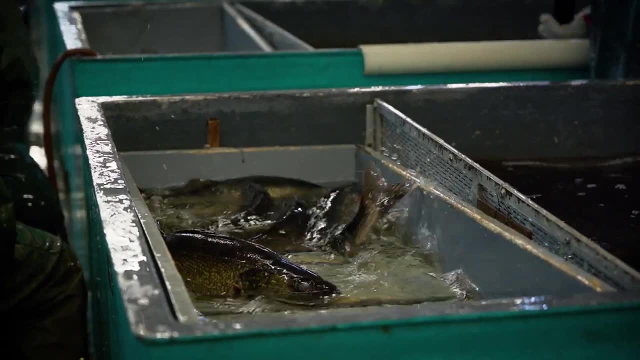 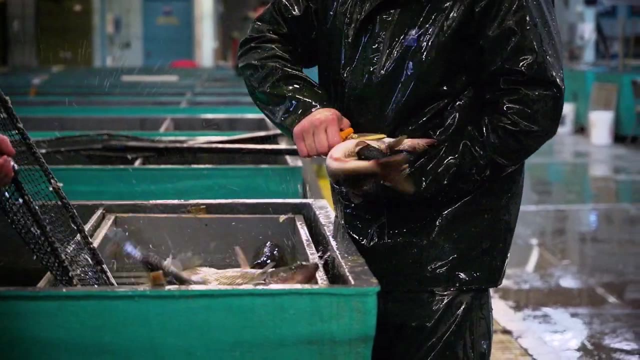 of fish. We're fortunate enough to have a great relationship with the hatchery here. when they're conducting their egg take, they have access to between 15 and 20,000 fish every spring and they allow us to mark those fish during their process. To mark them, we cut off a fin. this is not. 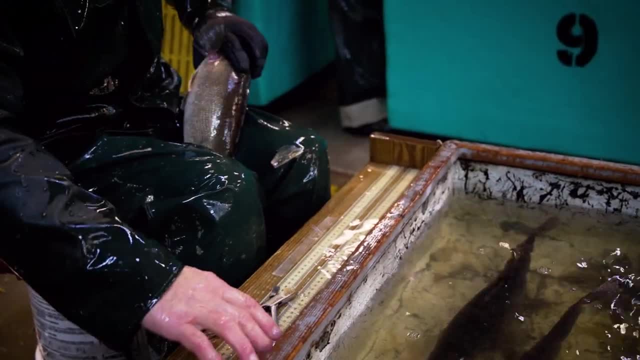 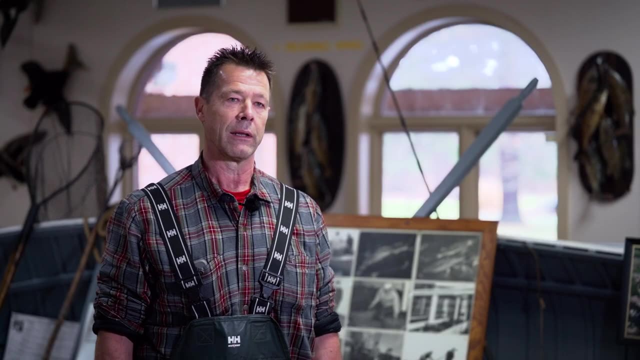 detrimental to the fish. we've done experiments in the past where we mark fish in a similar way and hold them in ponds, and we have 100% survival. The fin eventually grows back, but we can identify a clipped fin at least once a year. The fish that are in the lake are usually the ones that are 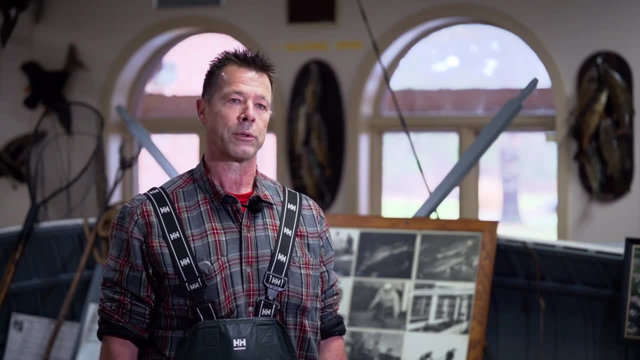 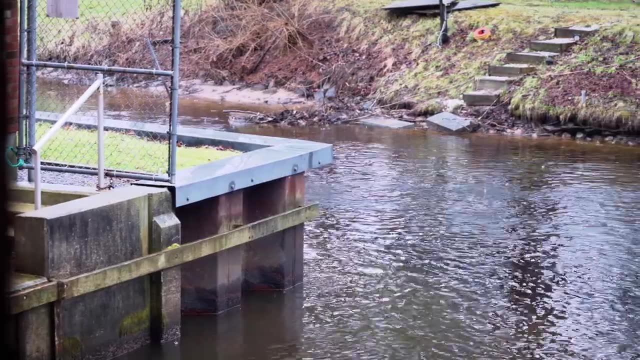 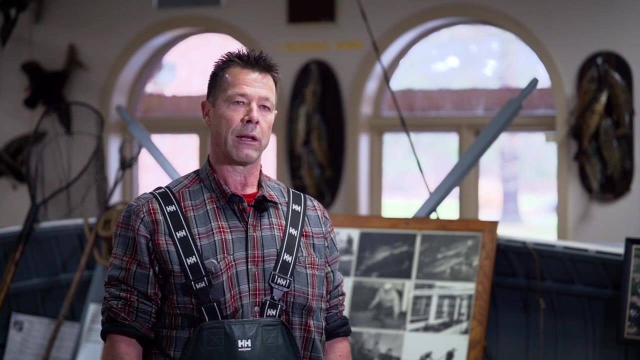 released through the first year, which is all we need for a marker capture. That's an old fin clip that's from three years ago. So after the fish get marked they're released into the lake and they have about a month and a half of time to disperse throughout the lake and then in the 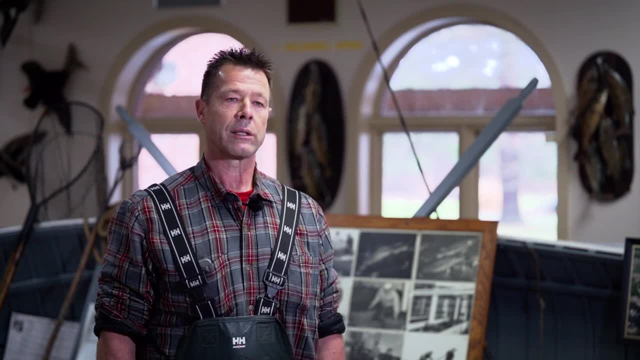 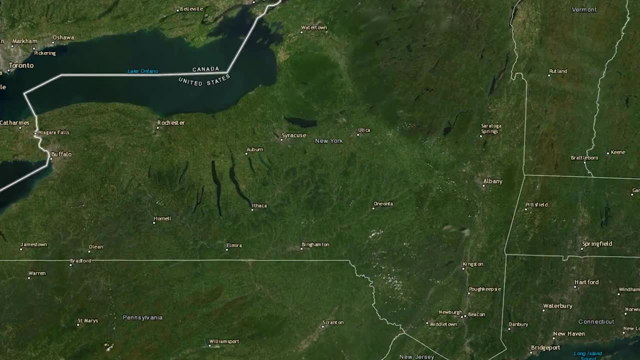 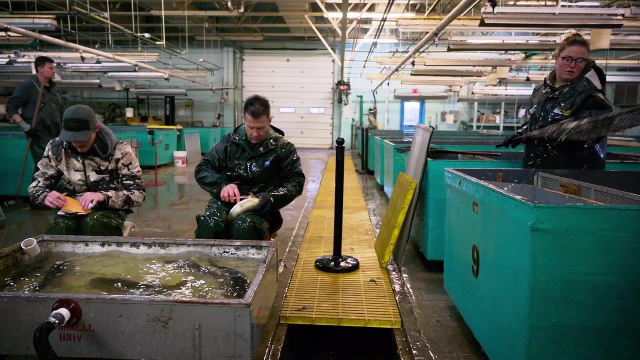 summer and fall we go out with our nets and sample as many fish as we can, and the ratio of marked to unmarked fish allows us to estimate the population. Oneida Lake has arguably New York's most valuable walleye fishery, and populations go up and down. Right now we're at about a million fish and 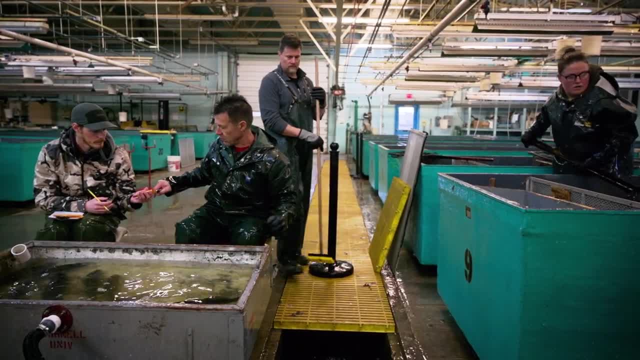 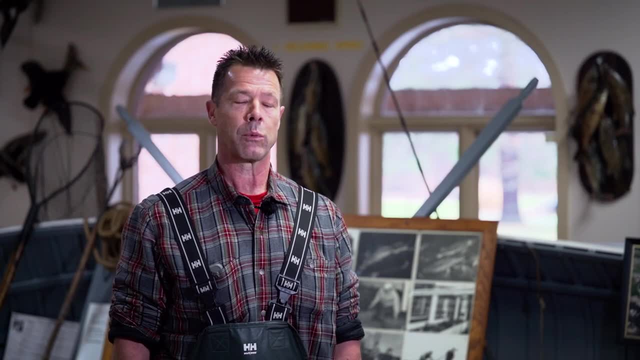 we've only seen that one other time. well, two other times, back in the 80s and then back in the late 50s. so we're really, you know, the population is really strong right now and we just want to keep tabs on it through marker capture every three years.